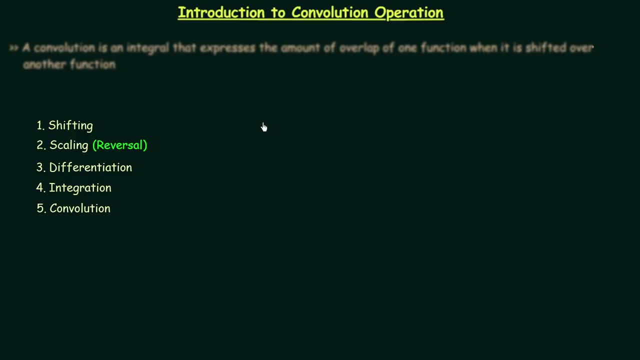 And now we can easily understand the convolution operation. Convolution operation can be used for different purposes, But in our course it is mainly used to calculate the output of an LTI system. So in this presentation we will see the definition of convolution, we will see the mathematical formula of convolution, we will see the number of steps involved in calculating the output using the convolution. And once we are done with all these things, we will solve one question. 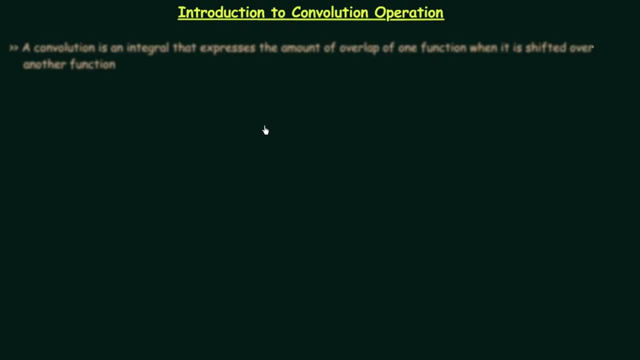 Which will explain all the steps involved in calculating the output using the operation known as convolution. And after this, before ending this lecture, I will show you the animation of convolution. So this lecture is very important. Initially you will find the convolution little bit confusing, But if you know the integration well- the integration I have already explained- if you know it well, you can easily understand the convolution also. So let's begin our discussion. 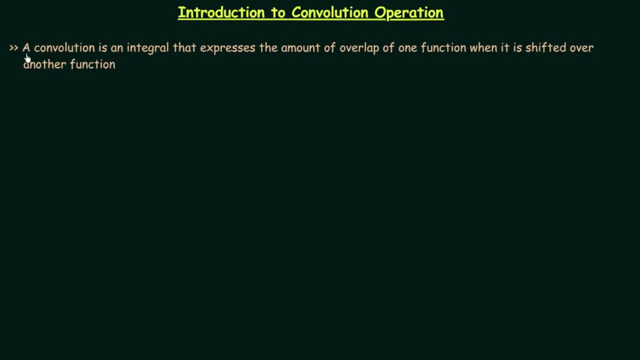 We will start with the definition of convolution. A convolution is an integral that expresses the amount of overlap- This is very important- the amount of overlap of one function when it is shifted over another function. So you can see five important points in this definition. The first point is integral. The second point is amount of overlap. 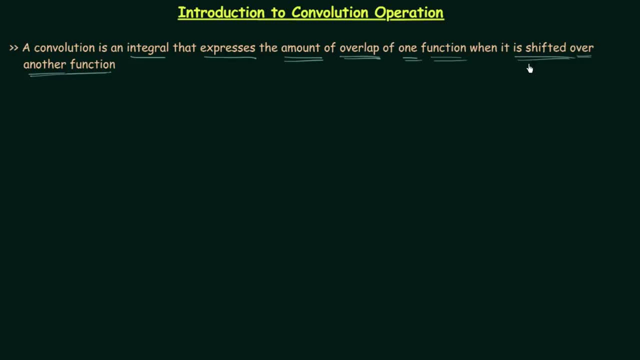 The third point is one function. Fourth point is shifted over and the fifth point is another function. So there are two functions involved. This is the first function. This is the second function. There is integration involved. There is amount of overlap involved when, when the function is shifted over the another function. This definition will be clear after solving one example. Now we will see the formula of convolution. 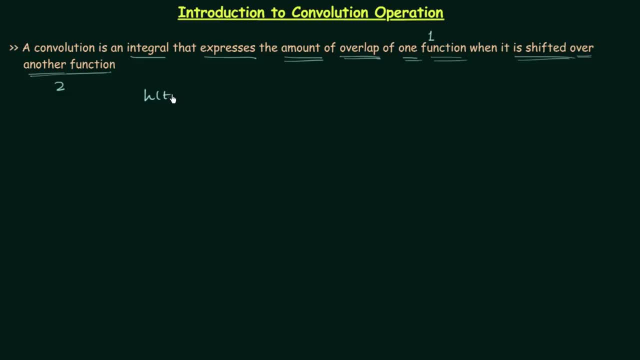 The impulse response ht of an LTI system is given and the input of the LTI system is also given, And now we are interested in calculating the output yt. So output yt is equal to convolution of ht and xt. So this operator here is known as convolution operator. 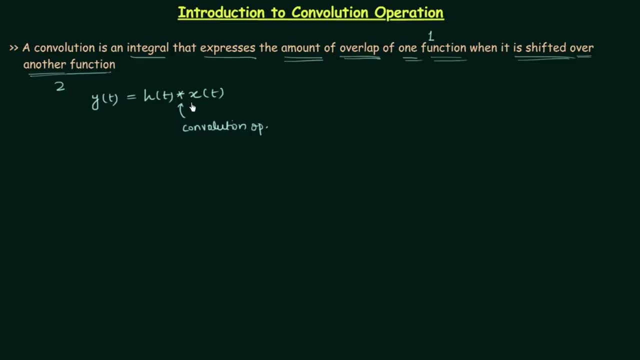 And the convolution operation between these two signals is equal to integration minus infinity to infinity: x tau multiplied to Ht minus tau d tau. So this is the formula of convolution And I will explain all the steps involved in performing the calculations using this formula. 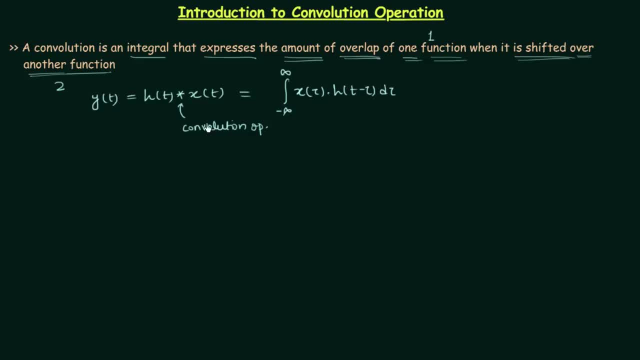 So we are having two signals. first signal is XT, the second signal is HT. so we have two signals: XT and HT. here we are discussing the different steps involved in calculating the output using the convolution. so in first step, we are required to replace T by a dummy variable tau. we will replace T by a dummy variable tau. we. 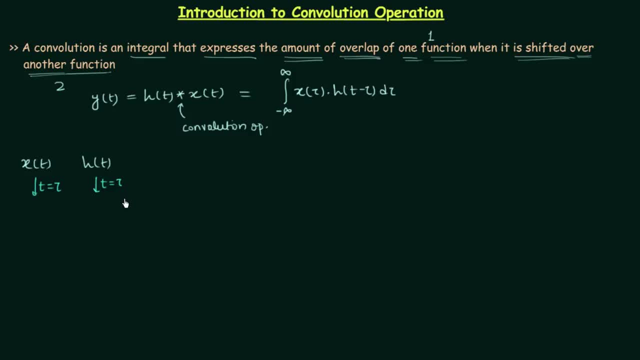 already know the reason to replace T by a dummy variable tau. we are going to move our signal, we are going to shift or move our signal waveform and for that we will vary the time T. so we don't want to confuse between the particular instant of time T and the variable time T we are having in. 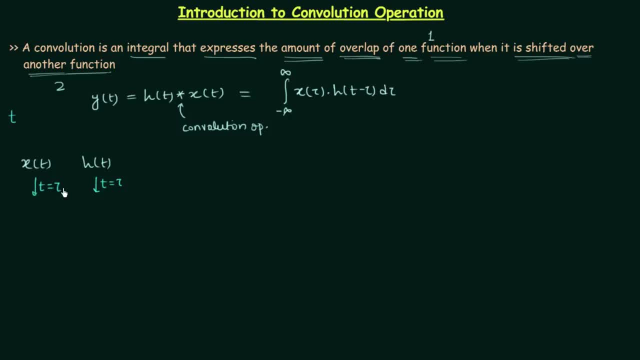 the signals. so it's good to replace T by tau. it will eliminate all the confusions while calculations are done. So we will have X of tau and here we will have H of tau. this is step number one. now we want one signal to get fixed, we want one signal to remain on its own position and we want X- tau to remain. 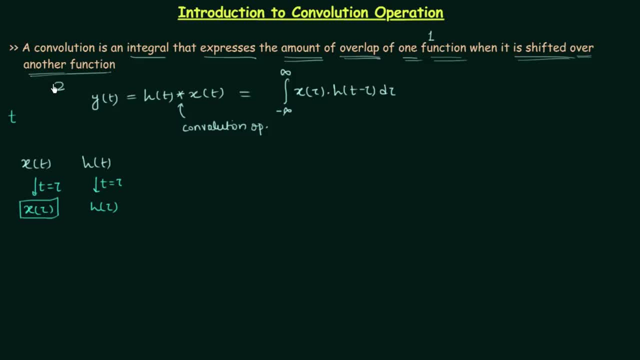 on its own position, because this another function here will remain on its own position and this function here we will shift and calculate the total amount of overlap. so we are interested in moving H T, which is now H aj, in S step number one, and for this we will first perform the time reversal. 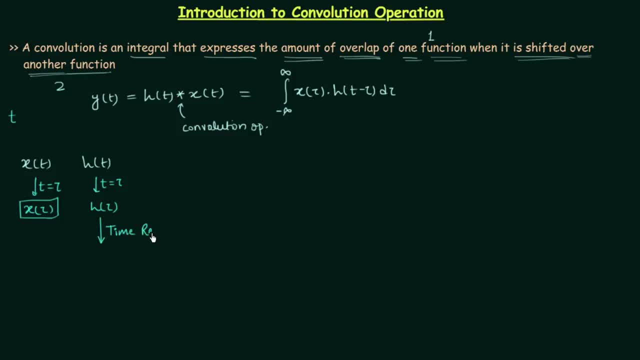 operation, the time reversal operation or you can say the scaling operation, and this will give us H minus tau. actually, we are implementing the formula written here, because using this formula we can easily perform the convolution will have our output yt. so we have x of tau, we have x of tau and we are trying. 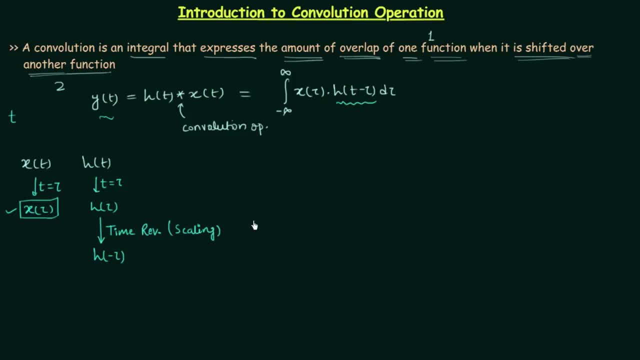 to get h, t minus tau. we have obtained h minus tau. now it's time to perform the time shifting. we are performing the time shifting operation and we know one important point related to multiple operations: the time scaling operation and the time shifting operation is only performed against the variable we are 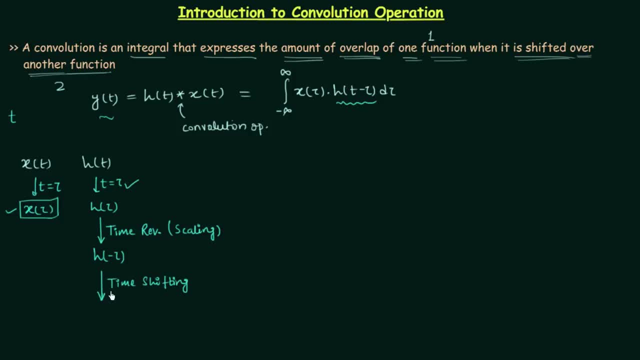 having the variable is tau, so we cannot perform the time shifting against minus tau. so it is important to take the negative sign out. we are having tau and here we will subtract T and when you simplify this you will have h t minus tau, the same thing we are having here. 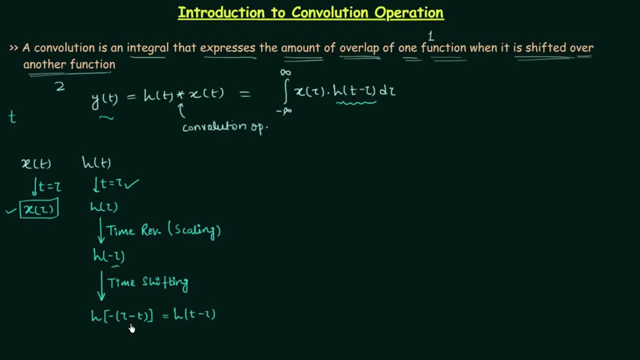 but this is the exact process we need to follow. we will perform the time shifting against tau because it is our independent variable. now it is a dummy variable which is acting as an independent variable. so we are done with time shifting. we have h t minus tau. we already had x tau and now we will. 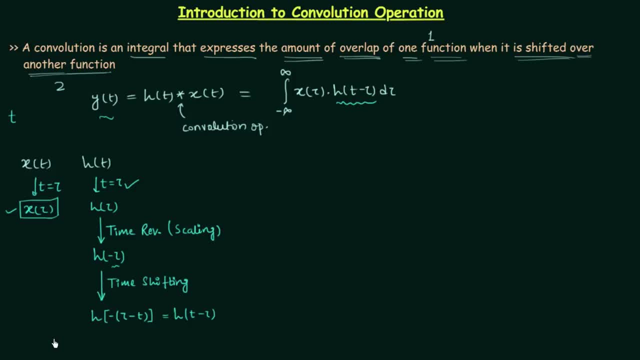 multiply them. we will multiply them, so we will have x tau multiplied to ht minus tau. and once you have the result of multiplication, you need to perform the integration. so from here we will have integration minus infinity to infinity: x tau multiplied to ht minus tau, d tau. so we are done with all the steps. the step number one is to replace T by 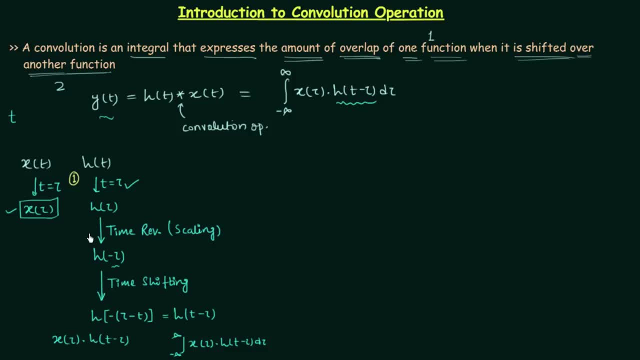 tau. we will have tau, we will fix it and then, in step number two, we will perform the time reversal. we will have h minus tau. in step number three, we will perform time shifting against tau. this will give us ht minus tau. the step number four is to multiply x- tau and ht minus tau. and the fifth step, the last. 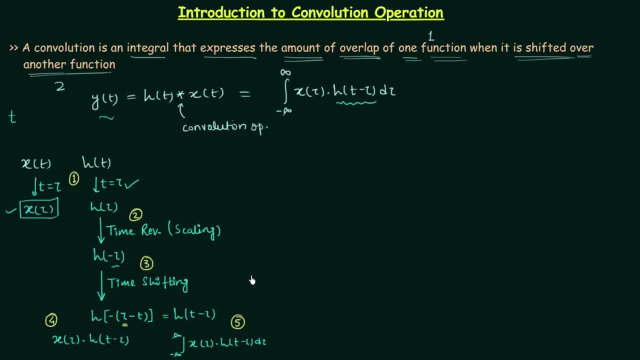 step is to perform the integration. so these are the five steps involved in the convolution operation, and now we will move to our example. in this example we have xt, the input of the lti system, and we also have ht, the impulse response of the lti system, and we are interested in calculating the output. 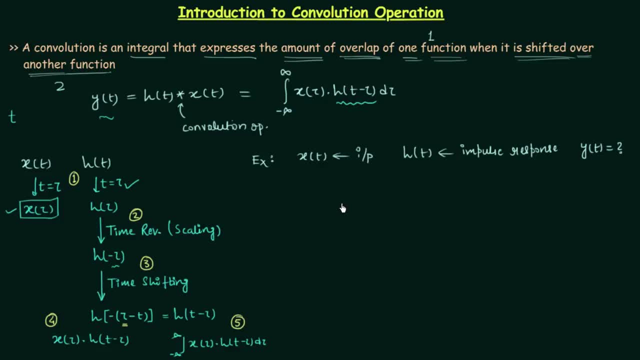 of the lti system and we are interested in calculating the output of the lti system, of the lti system. so i will quickly draw the waveforms of input and the impulse response. we are performing the graphical convolution here, following all the five steps. so let's see how the 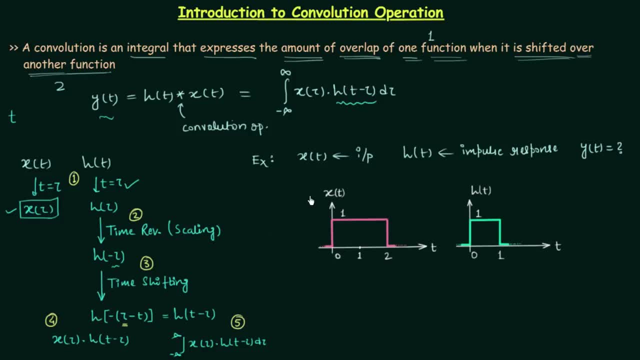 waveforms look. the pink waveform is the waveform of input, xt, and the green waveform is the waveform of the impulse response, ht. both are square waveforms, but the width of the first waveform- waveform of xt- is more as compared to the width of second waveform, the waveform of. 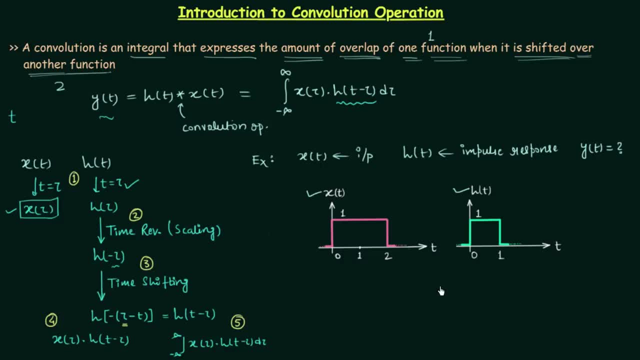 ht, and it is important to notice their widths, because we will obtain one important conclusion after obtaining the output yt. now we will perform our step number one, in which we will replace t by tau in both the waveforms. so let's quickly remove t and replace it by tau. 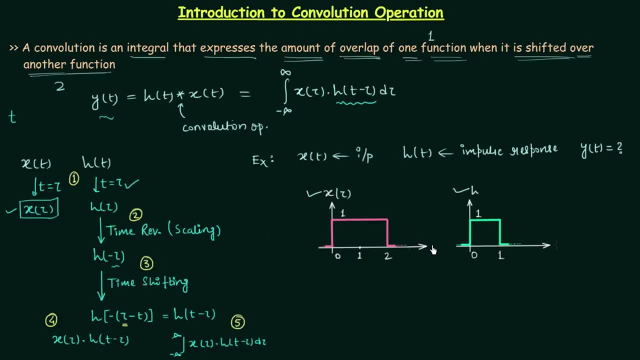 here we will have x tau tau, h tau tau. so we are done with step number one. now, in step number two, we will perform the time reversal, that is the special case of time scaling, in the signal h tau. we will keep x tau as it is and we will perform the time scaling, which is the time reversal to. 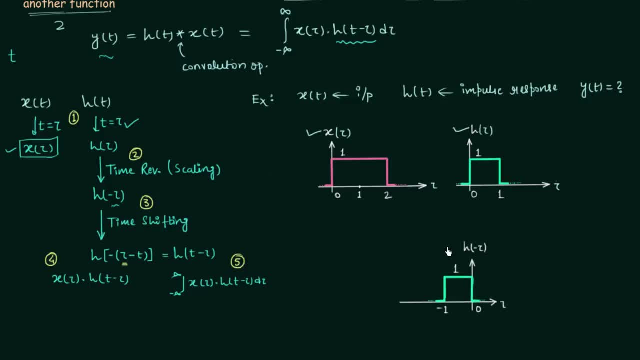 be exact. so this is how the waveform of h minus tau will look. we have simply obtained the mirror image about the y axis and this is the waveform. now we will move to step number three, in which we will perform the time shifting, and we know the process of performing the time shifting. I. 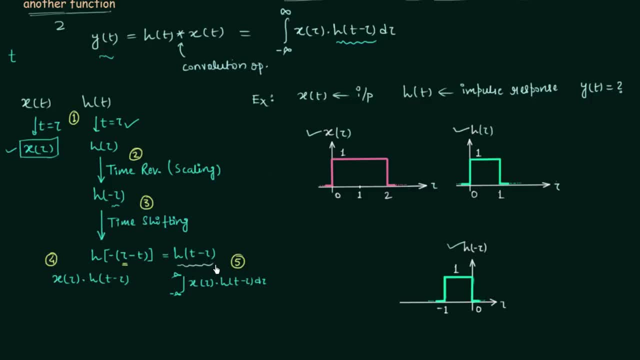 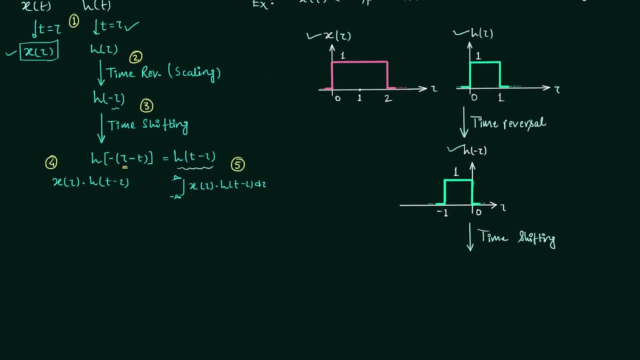 will directly plot the waveform of h t minus tau. but first let us mention that we have performed the time scaling or time reversal to obtain this waveform, and now we will perform. we will perform the next operation, that is, time shifting operation. I will quickly plot the waveform after performing. 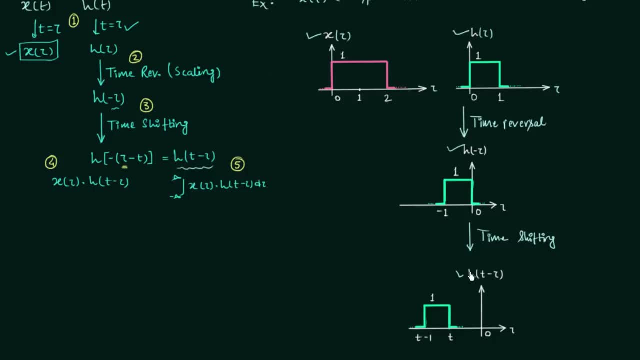 the time shifting. so this is the waveform of h, t minus tau. now don't confuse yourself that the towards the left y signal is not shifted towards the right because t can be positive or it can be negative. We will start performing the integration by moving our signal from infinity towards the 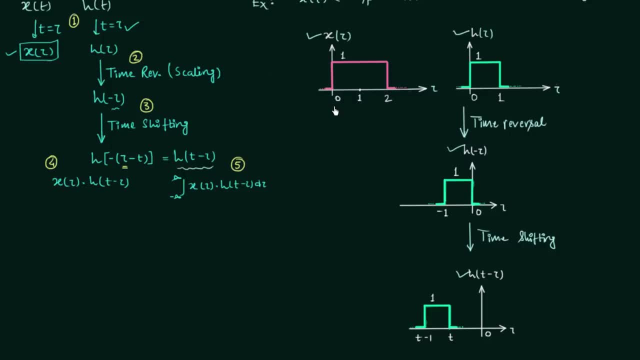 right, Our signal x- tau is non-zero from 0 to 2 and we will start moving our signal ht minus tau from infinity and we will calculate all the possible values of this integration. but it is smart choice to look for the time instance at which the signal value is changing, For example. 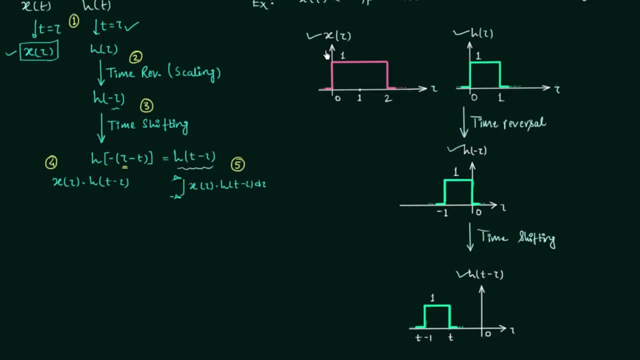 when tau is equal to 0, the signal value is changing from 0 to 1, and when tau is equal to 2, the signal value is changing from 1 to 0. So these points or time instance are very important to perform the convolution, because we don't want to. 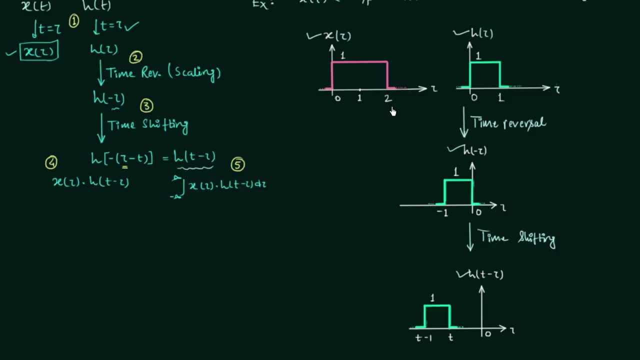 perform the convolution for each and every small increment in time. I will explain this in the next steps, but for now keep one thing in your mind: after performing the time shifting, this waveform can shift towards the right also, depending on the value of t, but we want to move our signal. 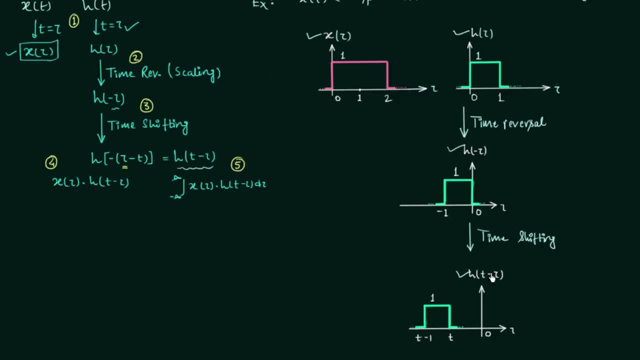 from minus infinity towards the right. so we are considering the value of t such that the signal is shifted towards the left. So this is all for step number three. Now we will move to step number four and step number five. We will perform step number four. 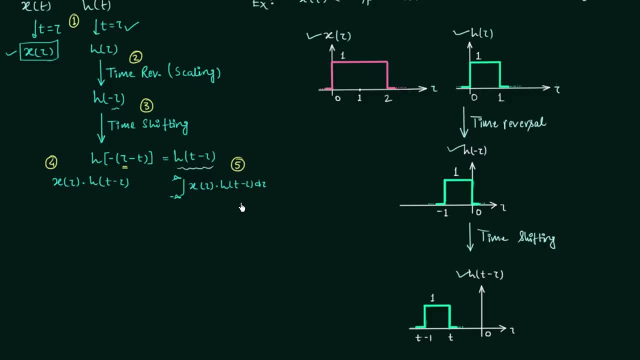 and step number five multiple times it is repeated. One, two and three are the steps we are required to do one time, but four and five will repeat more than one time. So let's see how we can calculate the integration by obtaining this multiplication. 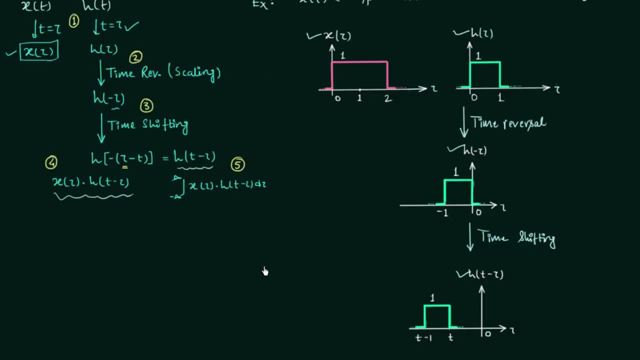 For this I will make another plot, which is the plot of x tau multiplied to ht minus t tau. in this plot, this waveform is the waveform of x tau and this waveform here is the waveform of ht minus tau, and we are moving ht minus tau from left. this arrow represents the movement of ht. 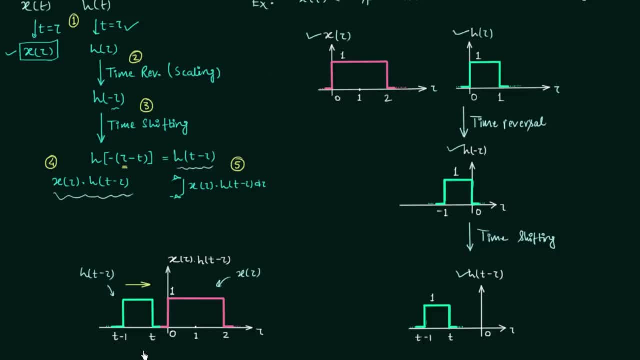 minus tau by the variation of t here. and you can see one important thing in the waveform of ht minus tau: when we shifted this waveform, the instant at which the signal value is changing from 0 to 1 becomes t minus 1, because initially it was minus 1. and when minus tau is replaced by 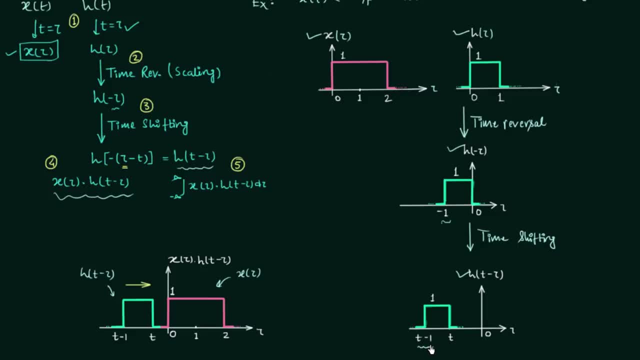 t minus tau, we will have t minus 1, and this instant here, which is the instant at which signal value is changing from 1 to 0, is 0. that's why we have t here. 0 plus t is equal to t, and this is important because when we shift this waveform from ht minus tau to ht minus tau, 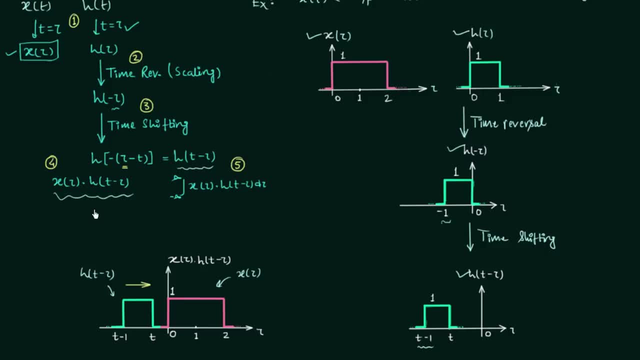 because we will use it while calculating the multiplication and hence the integration. let's say this case is case number one and in this particular case we are considering time t to be less than zero. here time t is less than zero. so you can see there is no overlap between the. 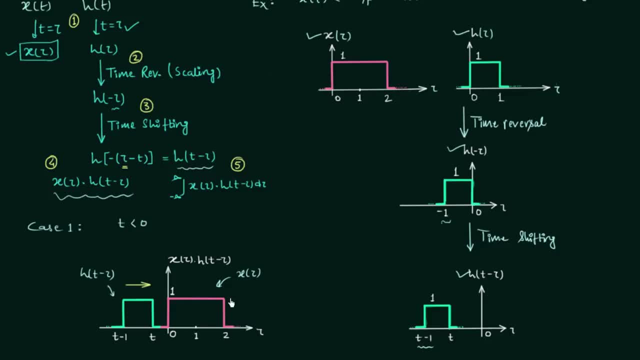 two signals: ht minus tau and x tau, and as there is no overlap, the multiplication is going to be zero. so we will have x tau into ht minus tau, equal to zero, and when you integrate it from minus infinity to infinity you will get zero. so i can write: yt is equal to zero. when t is less than zero, we are 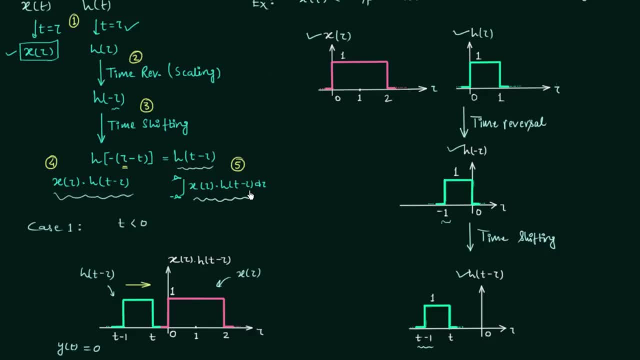